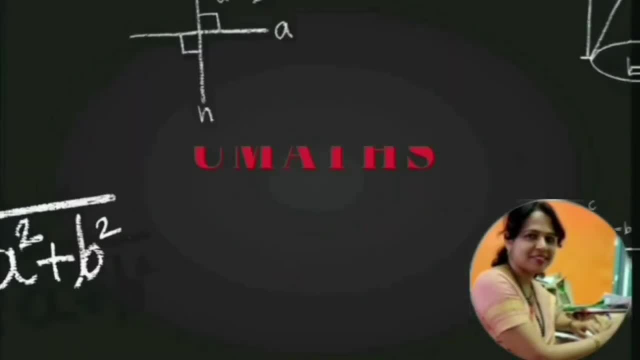 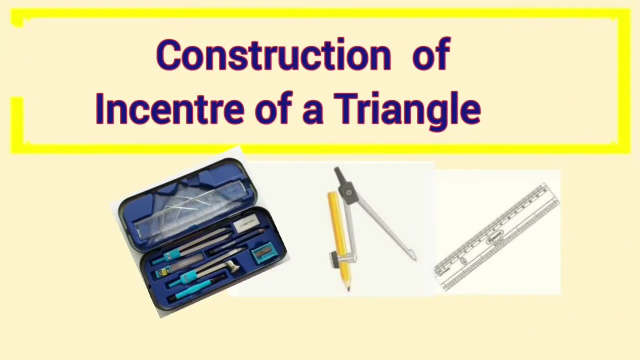 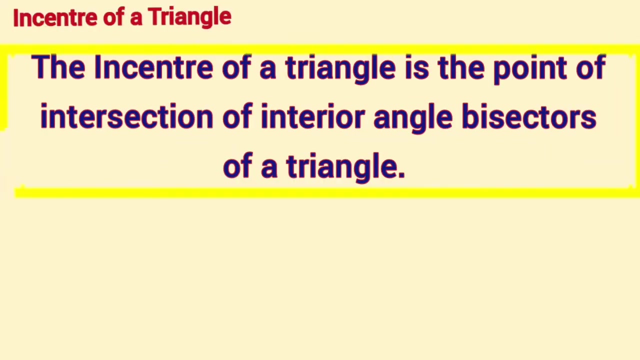 Hello students, welcome to U Maths class. I hope you all are eager to learn new concept with me. This video demonstrate how to construct in center of a triangle using compass and ruler. The in center of a triangle is the point of intersection of interior angle bisectors. 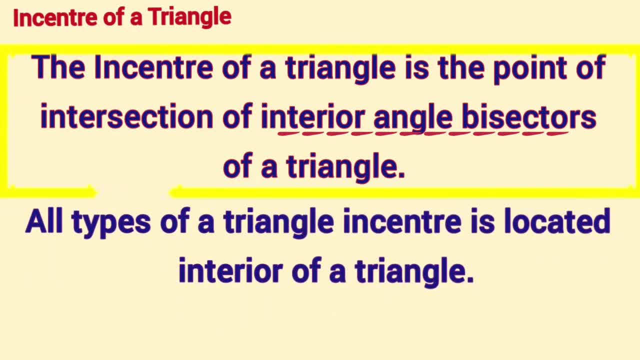 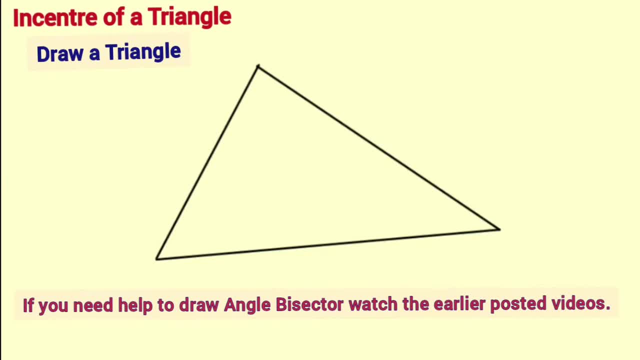 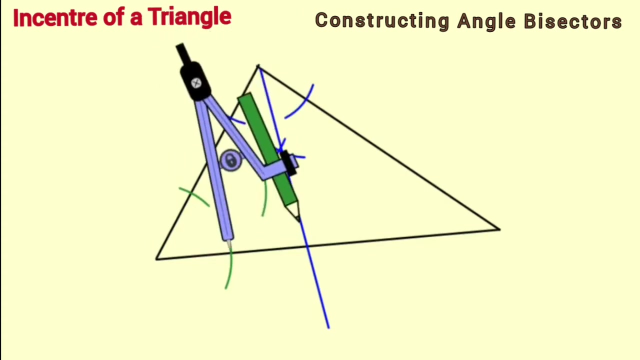 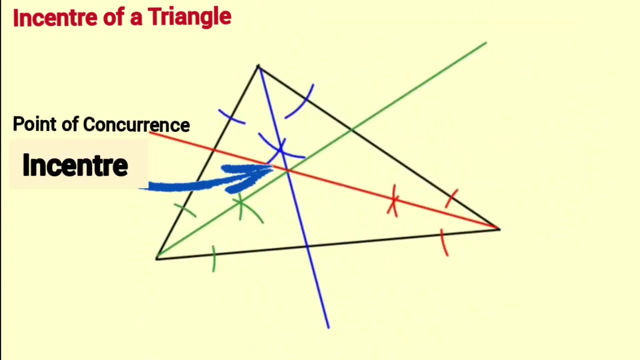 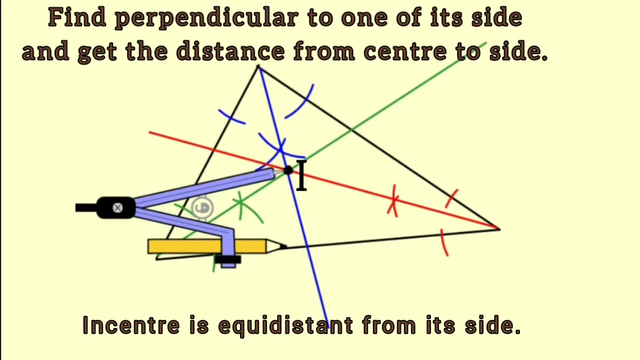 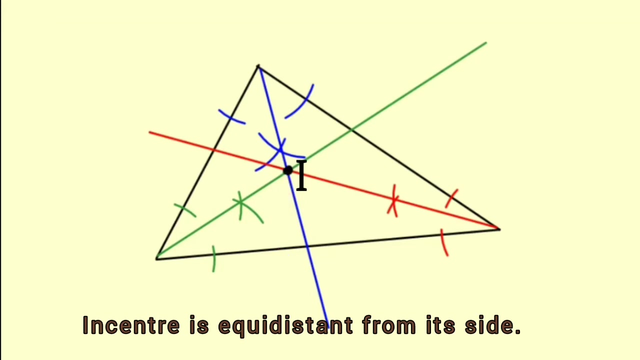 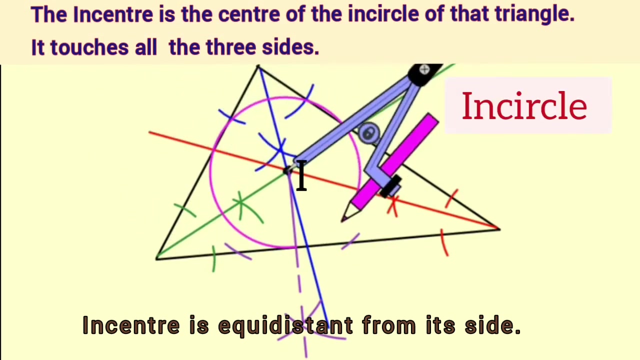 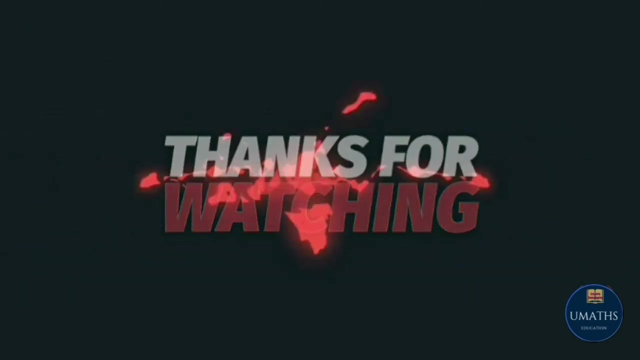 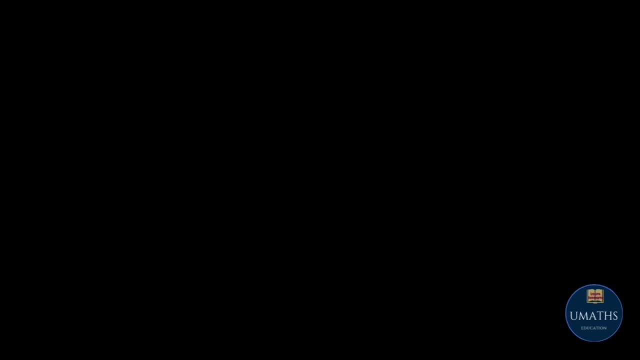 To get instant updates, subscribe my YouTube channel: YouMaths.